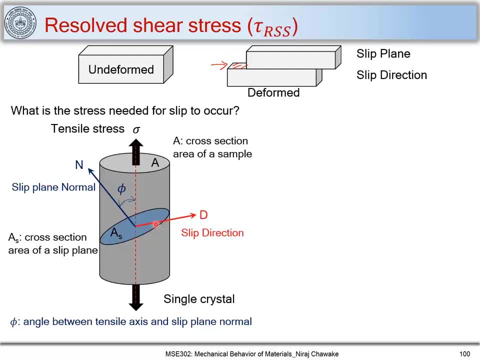 And let us mark A slip direction as D, which makes an angle of lambda with respect to our tensile axis. So this is a slip plane having area AS and slip normal N and slip direction to be D And the angle which they are making. the slip normal is making 5, angle 5 with a tensile axis, while slip direction is making angle lambda with a tensile axis. 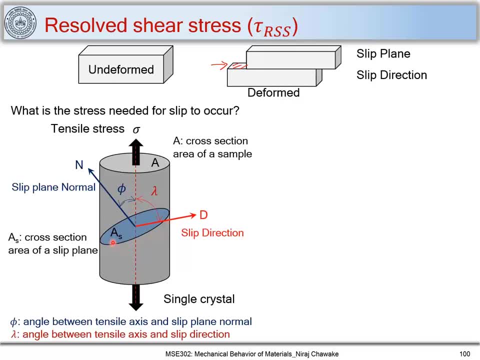 So this is how we define our slip system here. And let us say, I have this stress which is being applied. Now our aim is to find out what is a stress that is required to cause slip on this plane. That is our aim. So we have to find out a stress with respect to the applied stress, that is, a tensile stress. 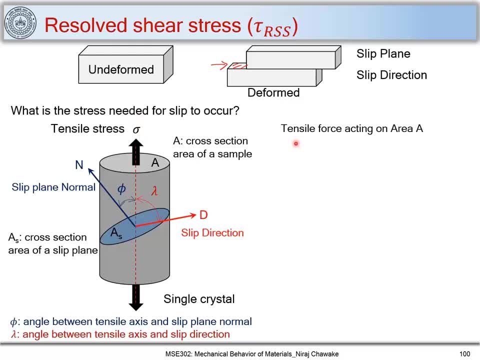 And let us do that. So first thing which we do is like find out a tensile force acting on area A. Let us find out the force F acting on this area A, and that is given as F is equal to sigma A. Now we know that slip occurs along the slip direction. 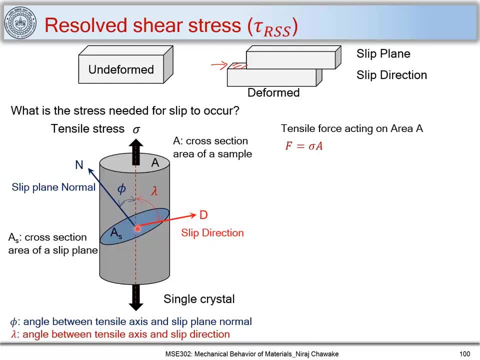 So let us find out a force which is acting along the slip direction. So to find out that we have to find out a component of F along slip direction. So FD is equal to F cos lambda, So it makes an angle lambda with slip direction. 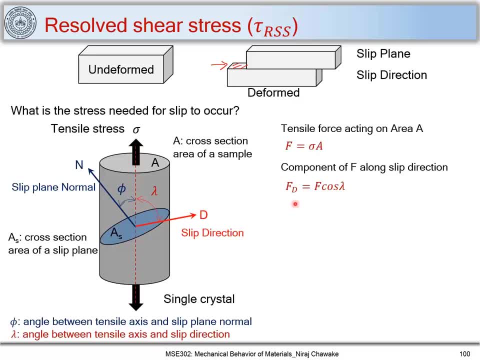 The tensile force is making an angle lambda with slip direction, So I can write it as: FD is equal to F, cos lambda. Now we have to find out a shear stress which causes slip to occur, So we call it as a viscous stress. 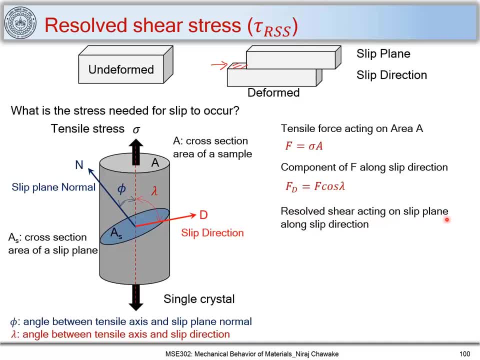 So I call it as a resolved shear stress. acting on a slip plane which acts on the slip plane along slip direction. So you can find it out by dividing the area of this slip plane. So let us do that. I call it as this resolved shear stress. has to be tau RSS and it will be given as FD upon AS. 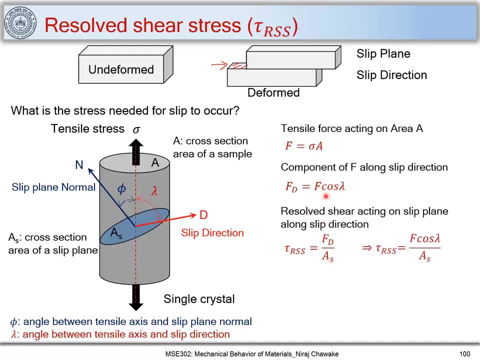 Now I put this value here of FD, Which is nothing but F cos lambda, And I get tau RSS to be F cos lambda upon AS. Now you can also find out AS in terms of A, which is given as A upon cos phi. So this plane, that is a slip plane, and the normal to this slip plane is n. 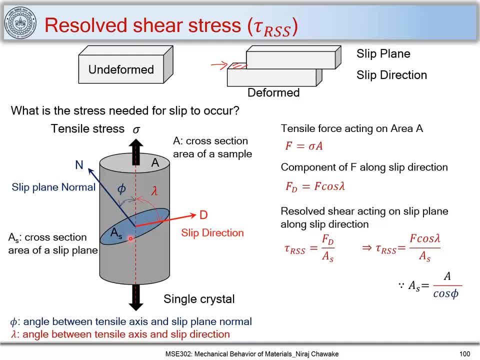 Which is making an angle phi with respect to tensile axis, And using this geometry you can find it out that AS must be equal to A upon cos phi. Now, if I put this value of AS in this relation, You can say that tau RSS to be equal to F cos lambda into cos phi upon A. 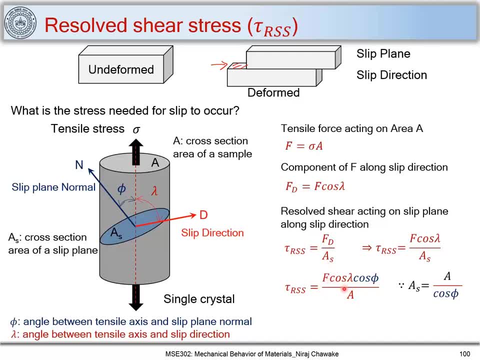 So if you look at this relation, I can replace this F upon A by sigma using this relation, And let us do that So we get this. We get tau RSS, that is resolved. shear stress acting along a slip direction on a slip plane Equal to sigma. cos lambda into cos phi. 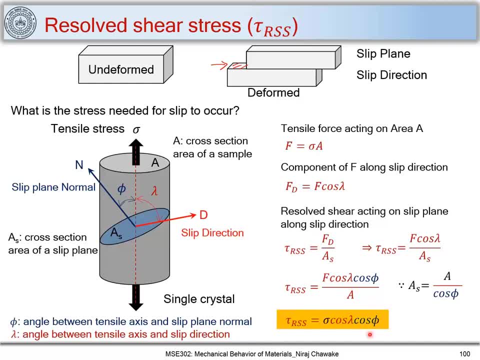 So this is a relation. This is simple but very important relation. By this relation you can relate the tau, RSS, that is a resolved shear stress acting on any slip plane, With applied stress, normal stress, that is sigma And, if you know the angle, lambda and phi. 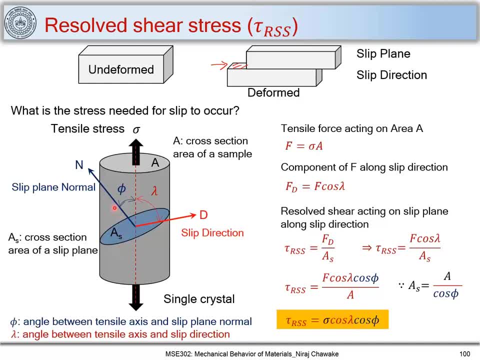 Which are the angle this slip system is making with the tensile axis. So this relation, we can use it to find out what is the resolved shear stress on any given plane. Now let us move on and see the implications of this relation. So we have this relation. 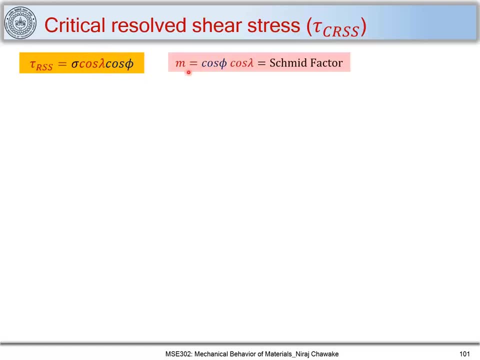 Where I replace this cos lambda into cos phi as m, And this is called as a Schmidt factor. There are two special conditions or situations which I would like to discuss. So let us consider a single crystal here. And the tensile axis is marked. 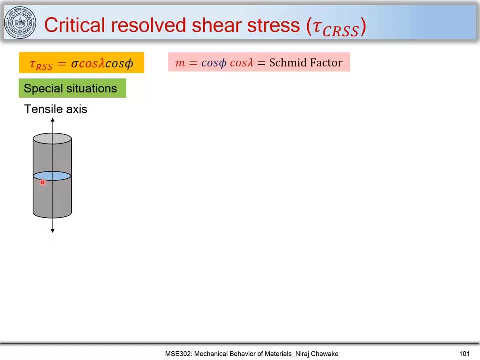 And let us consider this slip plane to be perpendicular to tensile axis. Now, in this case, if I see a D, which is a slip direction, You can clearly see that Lambda will be equal to 90 degree, Which is nothing but an angle between a tensile axis and the slip direction. 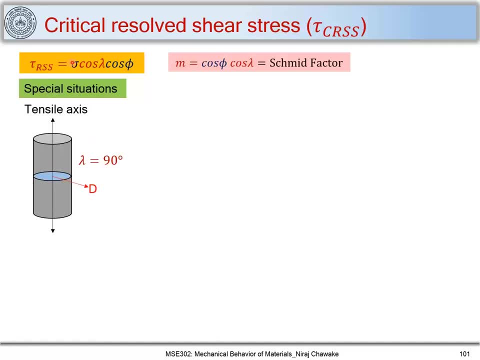 So it comes out to be 90. And if I use this relation, What the value of tau RSS you get is equal to 0.. Now, similarly, you have another situation Where your slip plane is parallel to tensile axis. So this is one extreme. 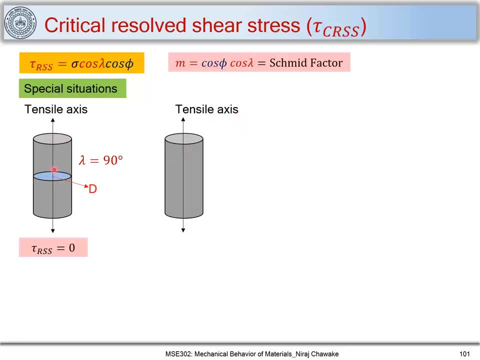 Where the slip plane is perpendicular to tensile axis. And this is another extreme, where the slip plane is parallel to tensile axis And in this case if you draw a slip normal, A slip plane normal, And you can say that phi equal to 90 degrees. 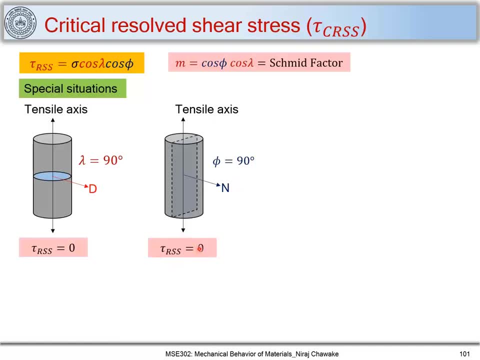 And the tau RSS comes out to be equal to 0.. So you can say clearly that for these two extreme cases, Where slip plane is perpendicular to tensile axis And slip plane is parallel to tensile axis, That there will be no shear stresses on these two planes. 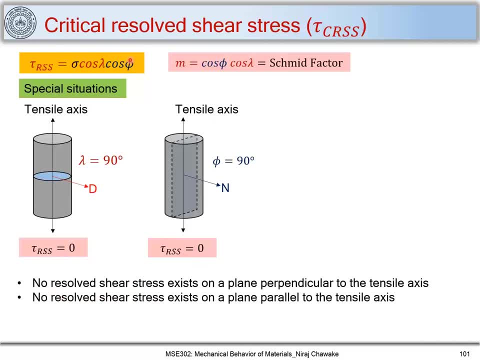 Now let us look at this relation in more detail way. So I have tau RSS equal to sigma, cos lambda into cos phi And let us plot tau RSS versus sigma, So as you see that it is giving a straight line Where cos phi, cos lambda, which is a Schmidt factor, 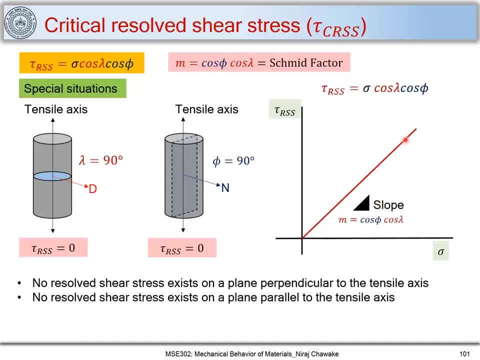 And will be a slope of this line. Now, as I increase the stress, The tau RSS is increasing And there will be a stage which will come When sigma, that is, an applied stress along the tensile axis, Reaches a yield strength of a material. 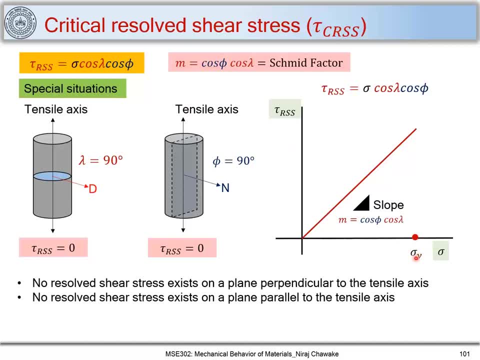 So let me mark that point over here, on the sigma axis as sigma y Now corresponding, there will be a resolved shear stress on a slip plane. So let us mark that point- And this point Is very crucial- Which is determining the slip. 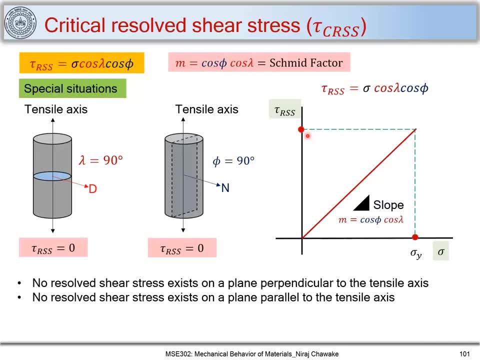 Slip phenomena which is occurring on the slip plane. So this point is called as tau shear stress, Or the shear stress which reaches on a slip plane corresponding to yield stress of a material Is called as critical resolved shear stress. Let me explain it to you again. 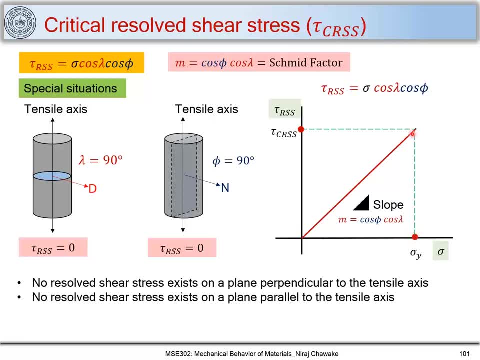 When material starts yielding, There will be a stress, Or a resolved shear stress, which will reach on a slip plane, Which will ultimately cause slip to occur, And that critical value of resolved shear stress is called as tau CRSS. Mathematical way I can say that as sigma approaches sigma y, 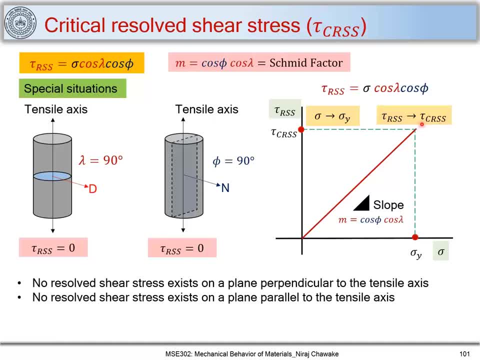 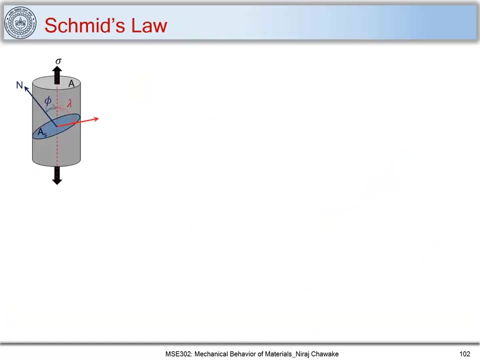 Tau RSS is reaching towards tau CRSS. So what is tau CRSS? It is the value of RSS at the point of yielding And is called as critical resolved shear stress. So this law, which was relating tau RSS with sigma And with this angle, is called as Schmidt's law. 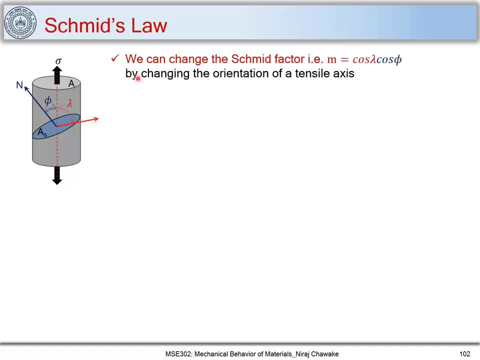 And let us look at this in more detail- We can change the Schmidt factor. So, if you see, mathematically We can change it by changing the orientation of tensile axis. So you can change this factor which is cos phi and cos lambda. 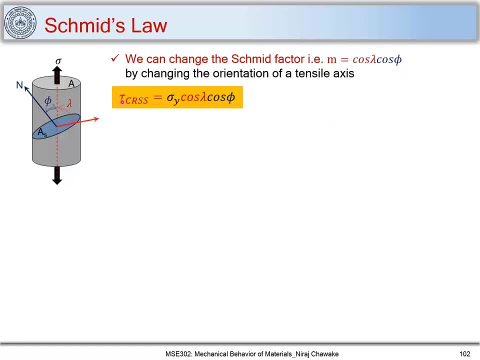 So if you have this relation, Tau CRSS, equal to sigma y, Cos phi into cos lambda, Look at this relation carefully. So when sigma has reached a value of sigma y, That is, yield stress, I write this tau as to be tau CRSS. 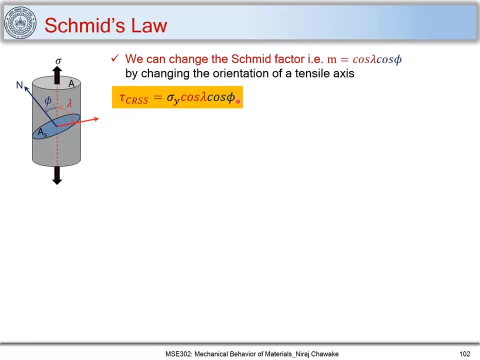 This is very important point To note. So here, mathematically, if you look at this relation, We can change this factor, cos phi and cos lambda, By changing the orientation of tensile axis. Now, at yielding this, equality must be satisfied. So you have three questions now. 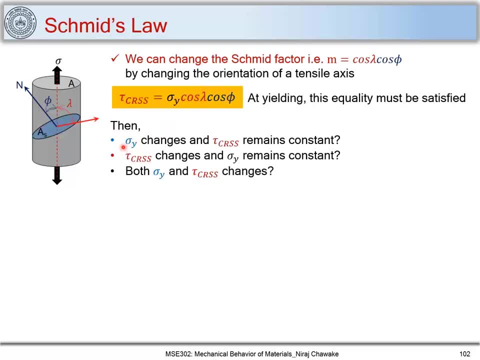 So when I can change this? So sigma y changes And tau CRSS remains constant. Or the second point may be: tau CRSS is changing And sigma y remains constant, Or both sigma y and tau CRSS is changing. So these are the three situations or three questions. 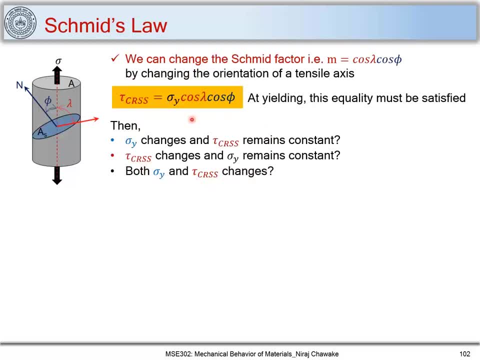 Which we can get from this relation. So which one is changing? That is what we want to find out, When we can change this cos phi and cos lambda. Which one is changing, Whether sigma y is changing or tau CRSS is changing? 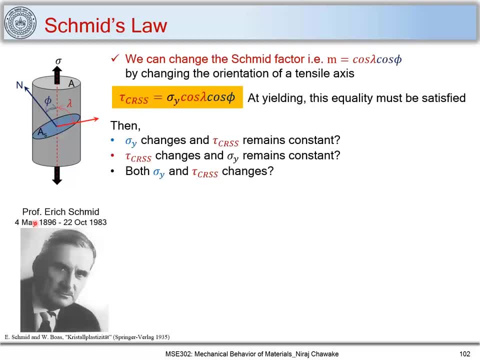 Or both are changing. Professor Eric Schmidt, based on his experiments or observations- This is called as Schmidt law, And he did very careful experiments And have seen that for magnesium single crystal, And he plotted tensile stress versus Schmidt factor, Which is cos phi, cos lambda. 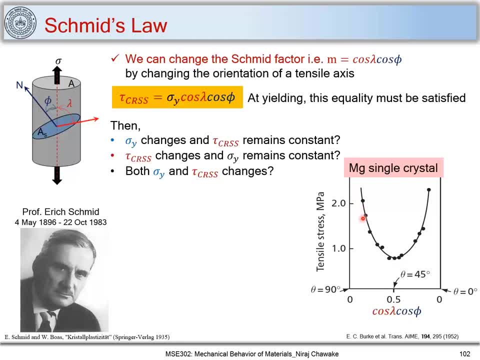 And he has seen that the tensile stress, Which is nothing but a yield stress, Is changing, Is changing with respect to cos phi and cos lambda And he proposed, with very meticulous experiments, That this value, that is a critical result, shear stress. 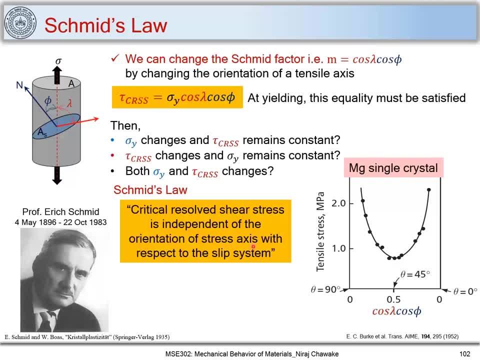 Is independent of the orientation of stress axis. With respect to the slip system, That means The critical result, shear stress, Doesn't change. It remains constant. The first option, that is, sigma y changes and tau CRSS remains constant, Is to be true. 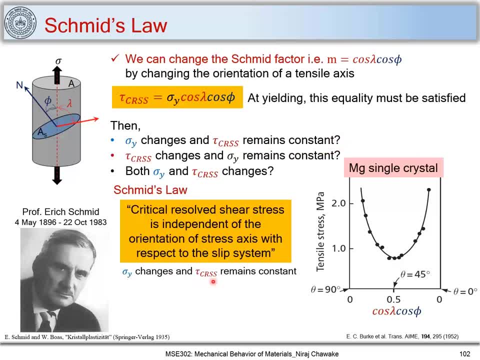 It is true. So sigma y changes and tau CRSS remains constant. This is a Schmidt law, So you have seen that. You can compare it now with anisotropic single crystal That if I have changed the orientation, Its yield strength changes. 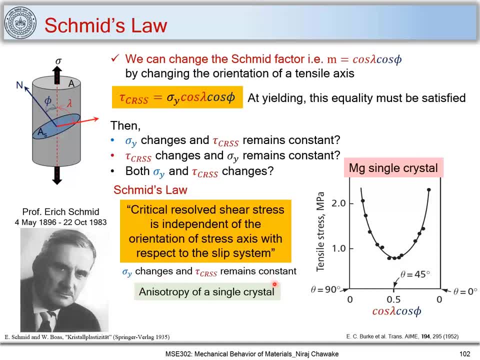 So this comes as an anisotropic single crystal. However, the tau CRSS. That is a critical result: shear stress Which causes slip to occur on a slip plane Along a particular slip direction. That remains constant Even if this cos phi and cos lambda is changing. 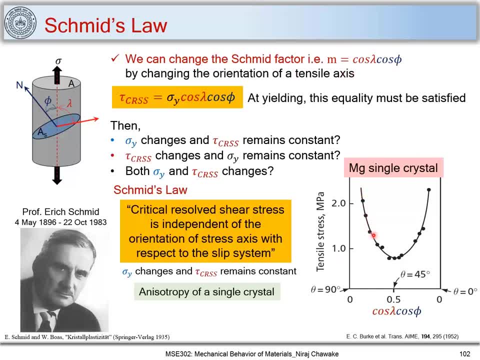 Or Schmidt factor, is changing. That is what is shown from this figure. So here you can see clearly That the tensile stress Is lowest at the highest Schmidt factor, That is 0.5.. Note this cos, phi, cos, lambda values as varying from 0 to 0.. 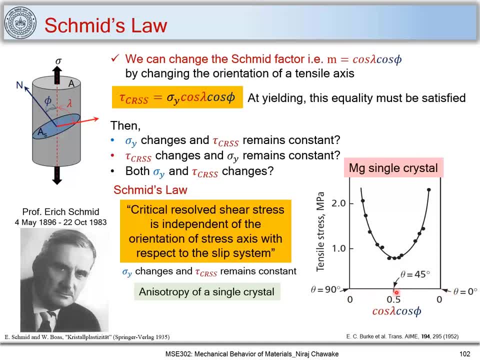 And the highest is at the center of this. So here you see that You get lowest value of tensile stress At the highest value of Schmidt factor, And that will occur only when That theta- Or here it is Phi and lambda. 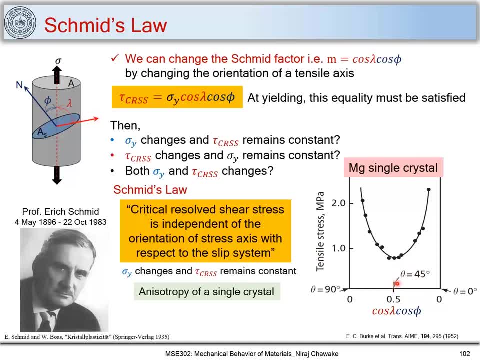 Are to be 45, 45. So which makes the highest Schmidt factor to come out to be 0.5.. Because cos of 45 will be 1 upon root 2.. And here, if I put 1 upon root 2 into 1 upon root 2.. 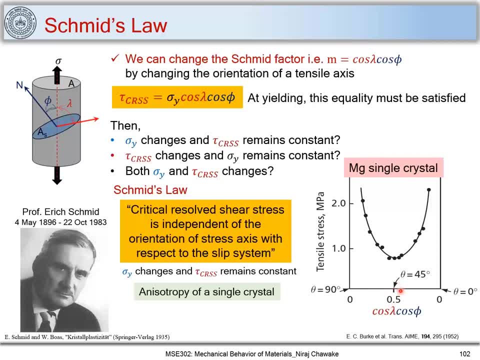 It becomes 1 by 2. Nothing but 0.5.. So you will have the lowest value of tensile stress, Or the material will yield at, Or yield at the lowest value of stress, And this Point is called as a soft orientation. 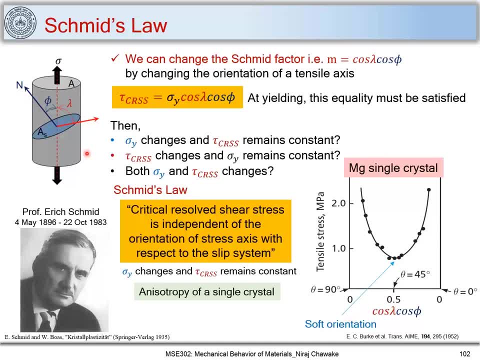 While if I orient my crystal in a way where The slip systems shows A lower value of Schmidt factor, Those are called as hard orientations. So let me write it down. So this part These are: These are Hard orientations. Similarly, these are hard orientations. 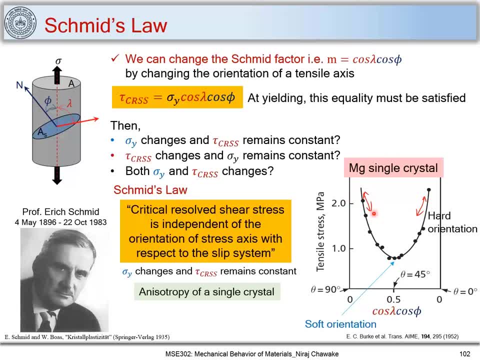 That means Material show Higher value of tensile stress, or yield stress, When they are Oriented Such a way that the Schmidt factor is lower. So here the point to be taken is that Material will show a lower yield value. 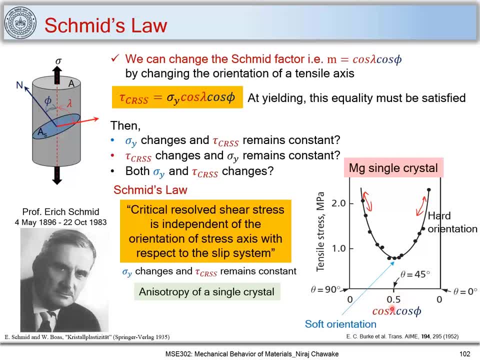 Or yield stress For Schmidt factor Which is a higher. So We can write it in a sentence That plastic deformation start on a slip system With the highest Schmidt factor. We have seen a different slip systems In material. So for a slip system, 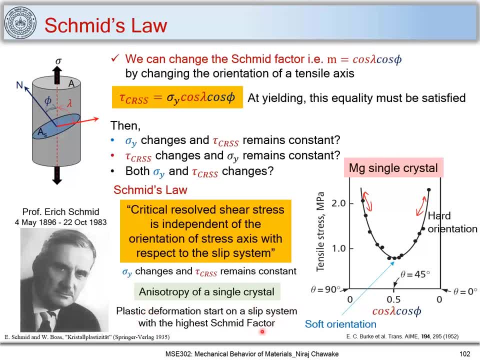 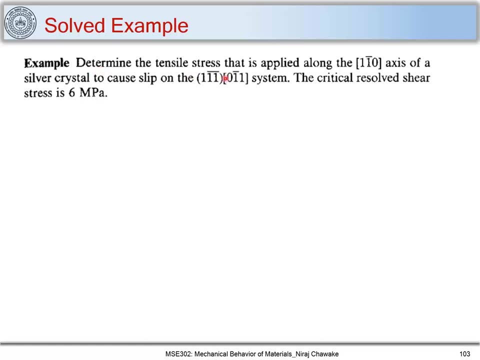 Where the Schmidt factor reaches the highest, Or is the highest, Will have Plastic deformation, will begin on that kind of a slip system. Now let's understand this by taking an example. Now let's consider This example. where determine the tensile stress? 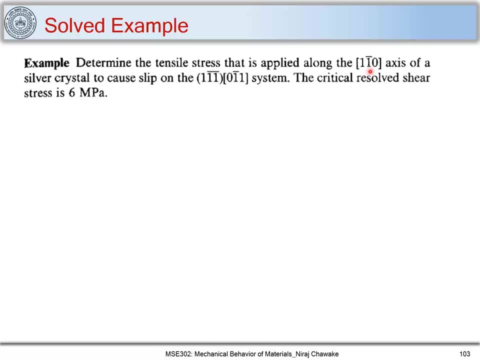 That is applied Along the 1, 1 bar 0 axis To a silver crystal To cause slip on the 1, 1 bar 1 bar 0, 1 bar 1 system. The critical result shear stress is 6 MPa. 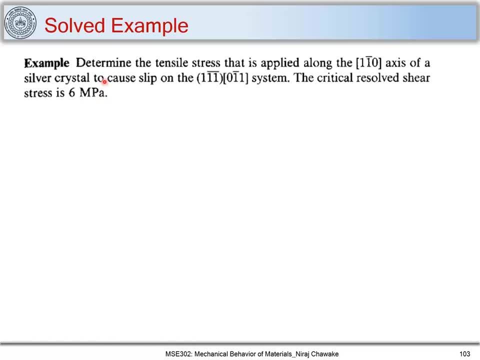 Let's read this question again Or try to understand. So we have to find out a tensile stress That is applied along. So you have given an Axis, tensile axis Along 1 bar, 1, 0.. For a single stress. 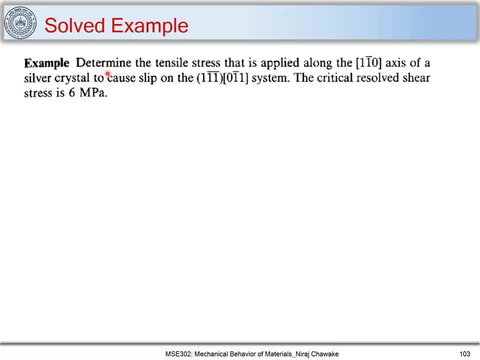 For a single silver crystal. So silver crystal is abscissive. So this is what an information you have to see, And the slip occurs on 1, 1 bar, 1 bar. That is this plane And this is a direction. 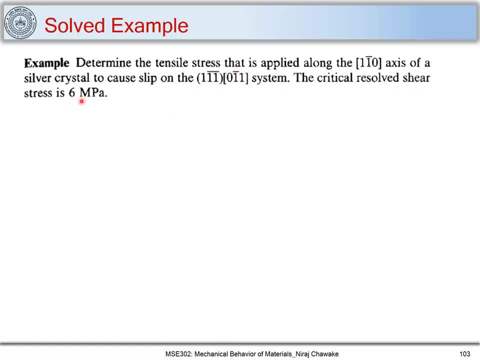 This is a slip direction. The critical result- shear stress, is given as 6 MPa. Let's understand this. So this tensile axis we have been given as 1, 1 bar 0. And you have given the slip plane. 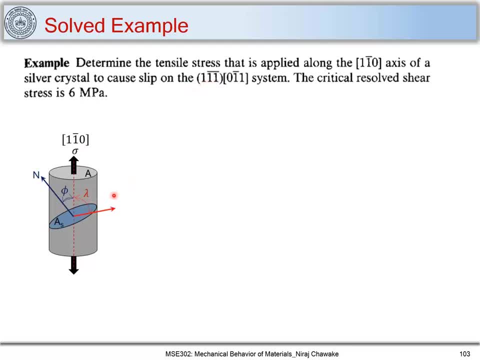 Which is like 1 bar 1, 1 bar, 1 bar. And this is a cubic system, So you can clearly say that the normal must be, Or the slip direction here is 0 bar, 1.. 0, 1 bar, 1.. 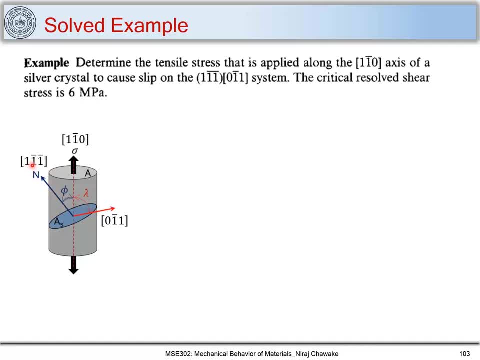 And this plane normal must be 1, 1 bar, 1 bar. So you can write it this for a cubic system. So we know What are the slip plane normal, Slip direction And a tensile axis. Now you can find out a angle. 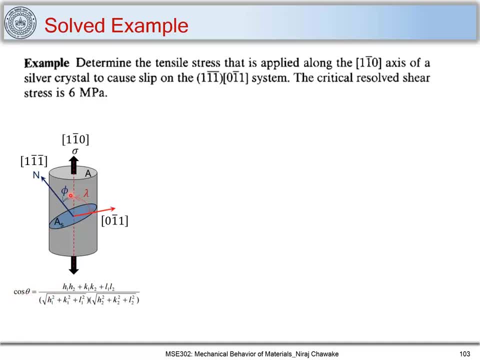 That is a cos theta Which you can see, that If I want to find out a cos phi Between slip plane, normal and tensile axis, We have to use- We can use this formula for a cubic systems And let's do that. 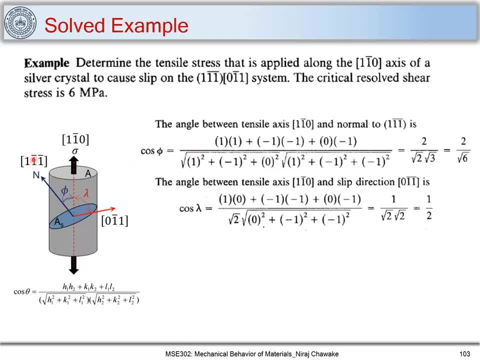 So cos phi will be an angle between Slip plane normal and a tensile axis And you plug in these values Here And you get cos phi equal to 2 upon root 6.. Similarly you can find out the angle Between tensile axis and the slip direction. 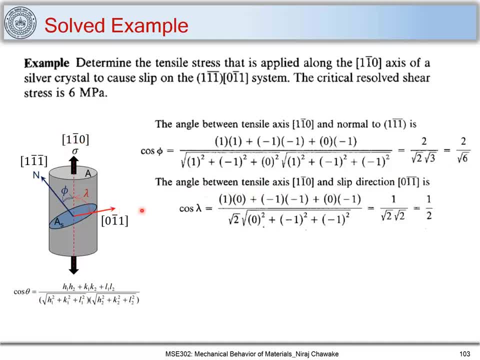 That is, this Tensile axis and a slip direction. Cos phi Comes out to be 1 upon 2.. Now We have been given The result, shear stress, to be 6 MPa, And from that What we have to find out. 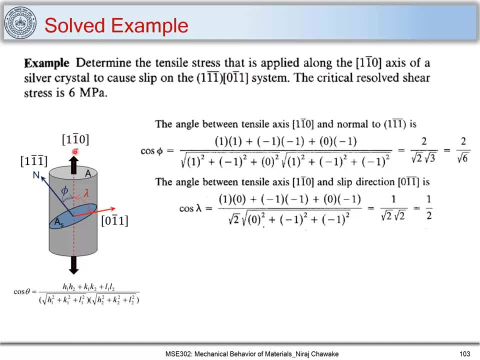 Determine the tensile stress That is applied. So we have to find out a sigma Which has to be applied. So we have been given Tau r And I have to find out a sigma, So which I write it as P upon a. 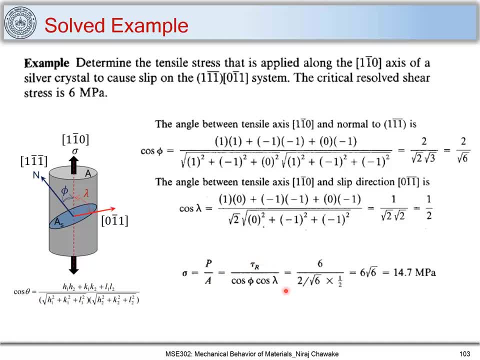 Which is nothing but a force upon area, And this relation we have already seen. So I get Tau r Upon cos phi. cos lambda Is equal to sigma, The value of tau r, That is result shear stress To be given as 6.. 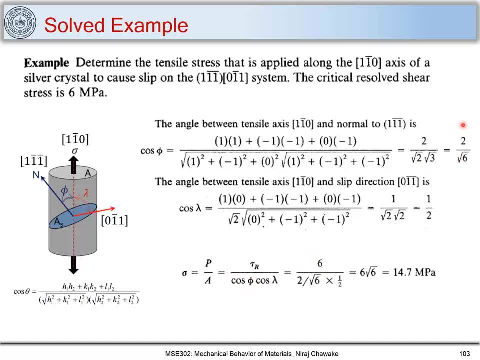 We have figured it out: Cos phi to be 2 upon root, 6. And cos lambda to be 1 upon 2. And you get a value of 14.7 MPa. If I know What is the result? shear stress. 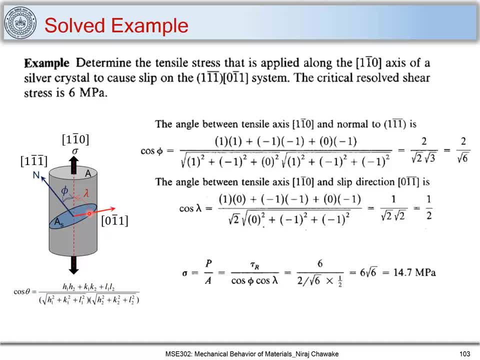 That is to be Needed to have a slip to occur. We can figure it out: What can be A stress That is required Along the tensile axis To cause this slip to occur. Or we can do vice versa If we know. 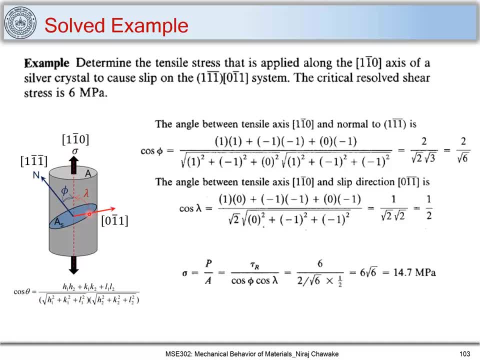 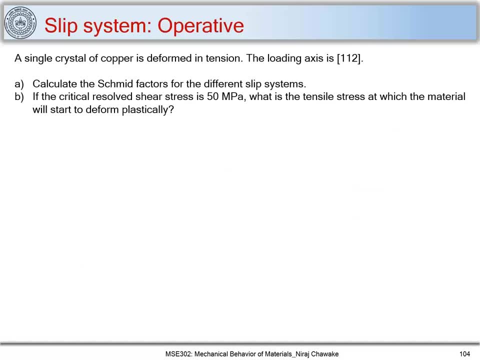 We know the stress. We can find out What is a Tau rss, Which is There on this slip plane. Now let's Let's consider this example To understand Schmitt law, Or Operative slip systems, In more detail. 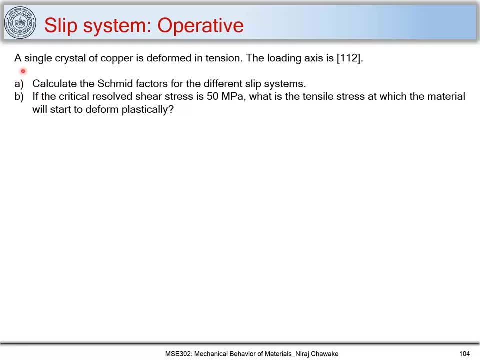 A single crystal Of a copper Is deformed in tension And the loading axis Is 112.. Calculate the Schmitt factors For the different Slip systems. For the different Slip systems: Calculate the Schmitt factors. 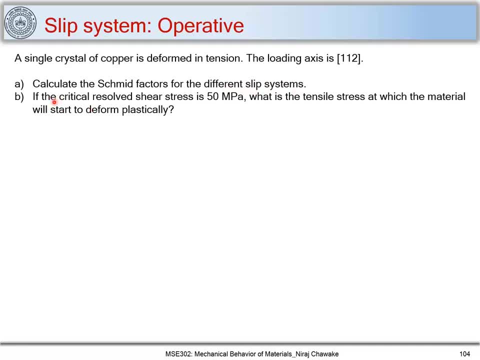 For the different Slip systems. If the critical Result- Shear stress- Is 50 mpa, What is the tensile stress At which the material Will start To deform Plastic? So let's read this And understand this question. 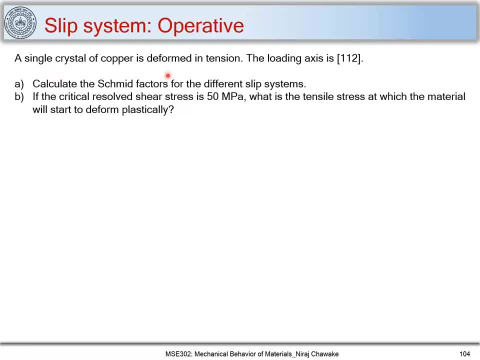 Again, A single crystal Of copper Is deformed In a tension. The loading axis Is 112.. So we have given A loading axis. Calculate the Schmitt factors For a different Slip systems. Now What are the different? 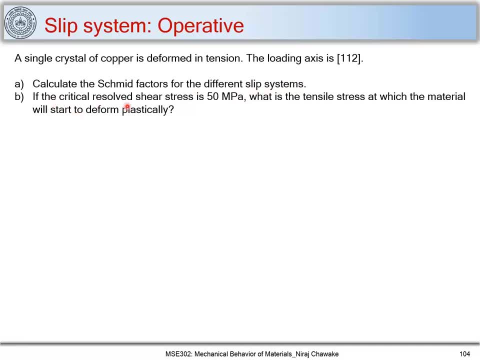 Slip systems. We have to answer This: If the critical Result- Shear stress- Is 50 mpa, What is the stress At which the material Will start To deform Plastic? Now, This is a copper. 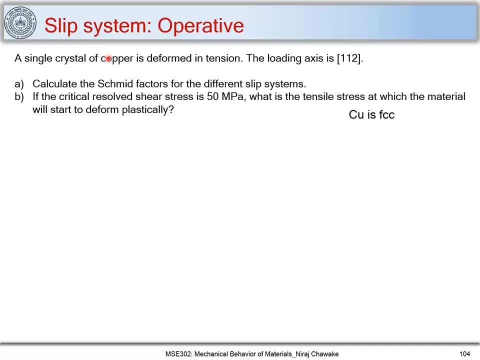 So you have an abscissive Crystal structure And Which has Copper, Is abscissive And the number of Slip systems Are 111.. That is A slip Plane And This is a 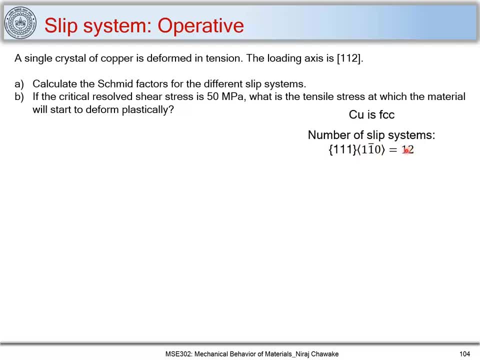 Slip direction. This We have already Seen. Now The question is Which Slip system Will be Operative. We have to find out, And We have seen that Slip system Will be Operative Where the 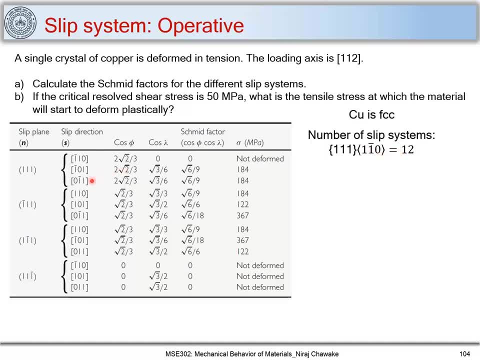 Schmitt factor Is Highest. Let's do that. Let's do Calculate All the Slip systems. So We have Slip Plane That is 111. And There are 4. Such Kind. 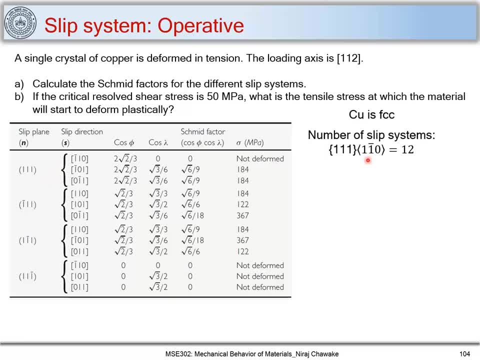 Of Slip Planes And There are 3. Directions On Each Slip Plane Which Makes To Be 12. Number Of Slip Systems To Be 12.. 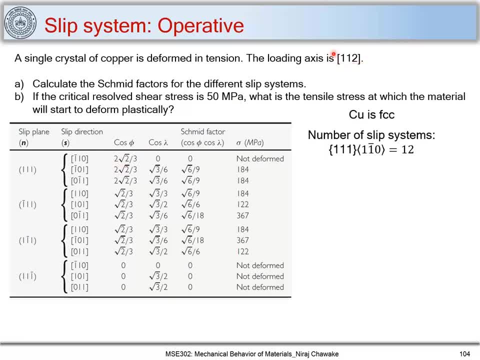 So Here, 3. Slip Plane Is Highest Slip Plane, So We Can Use This Relation That The Routing Axis Is Given As 112.. So Here, 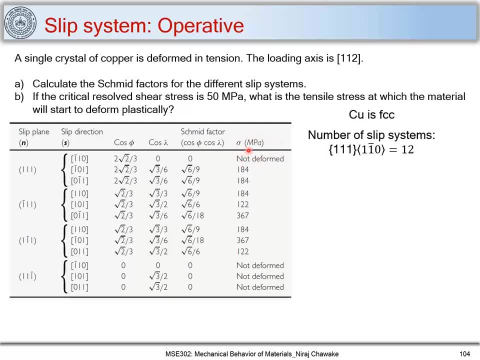 The Cos Phi Comes Out To Be 1.. Where This Plane, That Is, 1. Bar 1.. 1. And This Direction To Be 0.. 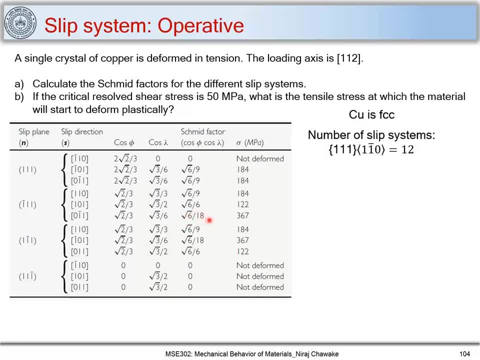 1. Bar 1. You Can See The Cos Phi Comes Out To Be 1. Bar 1. 1. And 1. 0. 1. This 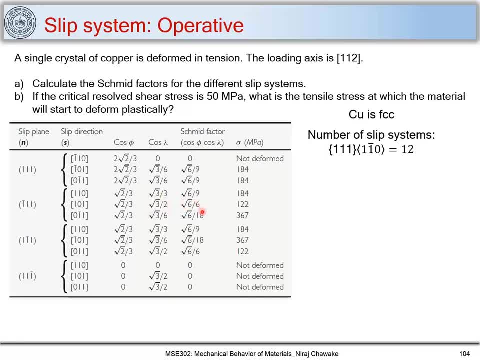 Like I Get A Cos Phi To Be Root, 2. Upon 3. Cos Lambda To Be Root, 3. Upon 2.. And See Clearly Here: 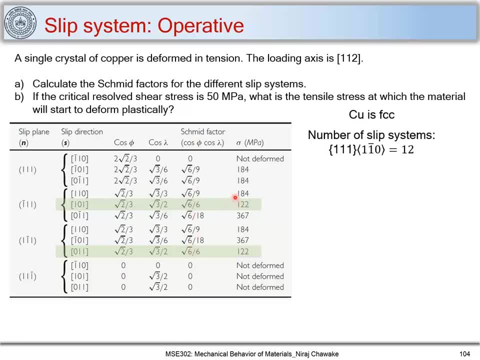 Root 6. Upon 6. Will Give You A Maximum Schmidt Factor, And Thus You Don't Need A Much Of Stress To Cause Yielding Or 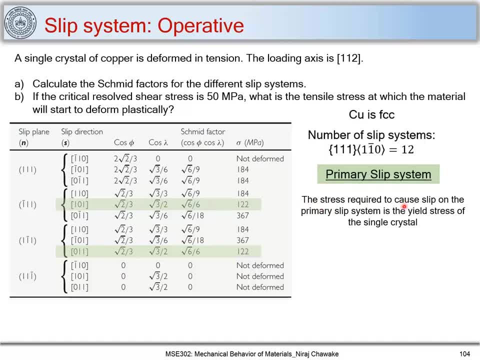 Cause A Sleep On These First Sleep On The Primary Sleep System Is The Ill Stress Of The Single System, And That Is What Is Being. 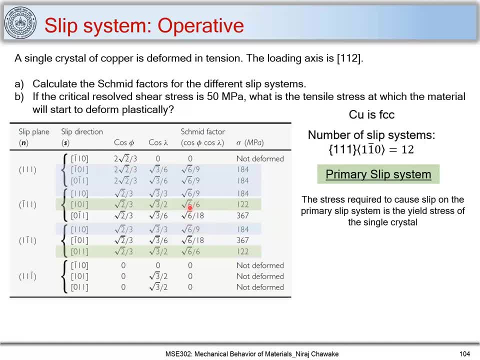 Defined. Now, If You See That This Was Secondary Sleep System, So As This Sleep System Will Start When The Load Is Increased Further And Then 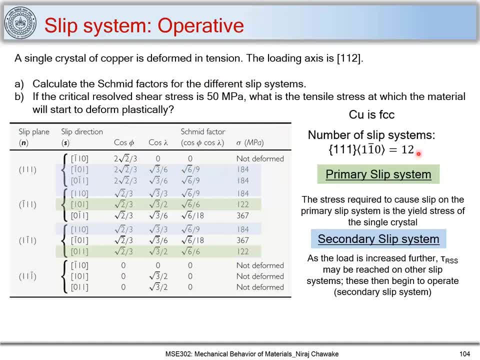 Towers May Be Reached On Other Sleep Systems And This Will Start As Me Factor. So Let Say, I Have This Single Crystal Which You Have. 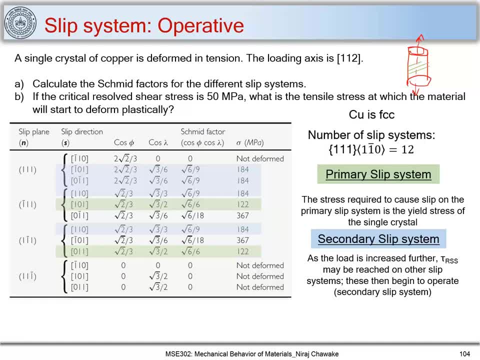 Seen Okay, And It Is Being Deformed And I Have, I Have Different. I Have Different. Sectional Is Highest Than The Green One. Let Me 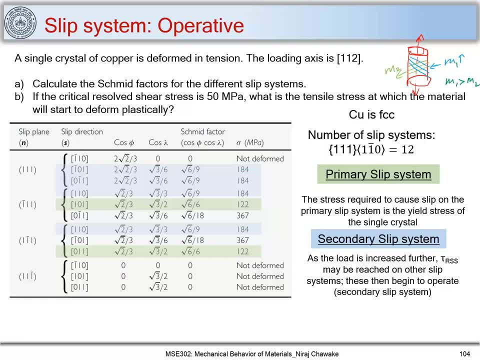 Call It As An Two And We Called This And One, So Time One Is Greater Than M2.. So What? to a certain level where the tau RSS will also reach on these planes, which are green planes. 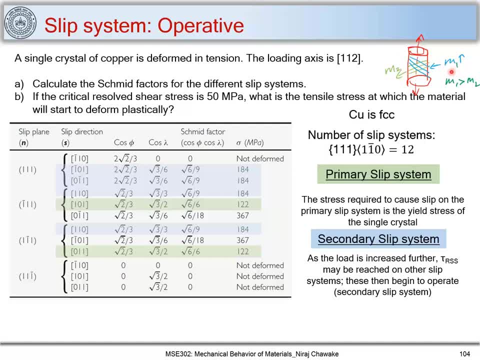 which has lowest mid-factor, as compared to blue planes, which has highest mid-factor. So slip will start occurring on the slip planes and then if we further increase load or stress, the slip will start operating on or slip will start occurring on these planes. So the blue ones will be a primary slip system which has the highest mid-factor, whereas the 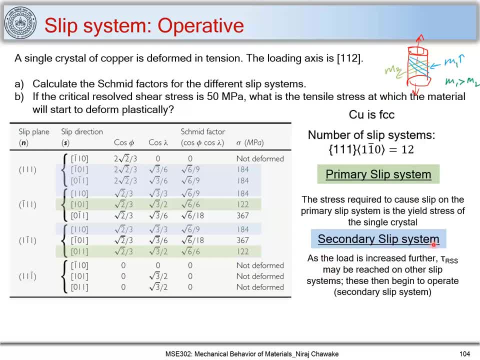 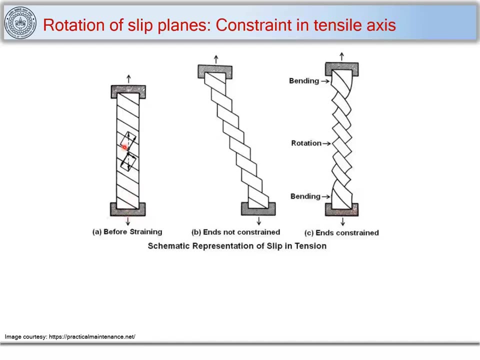 green ones are the secondary slip system, which has the lowest mid-factor, and with this example we have figured it out. what are primary slip systems and secondary slip system? So when we talk about slip, what we are doing is we have a single crystal. it is represented over. 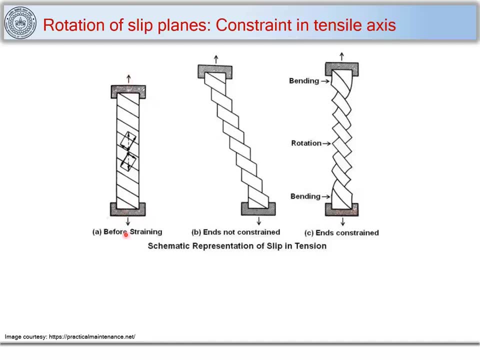 here. So when I try to put this single crystal under a tensile load or force, it will cause slip to occur. on a plane or a slip system where the mid-factor is the highest, When the ends are not constrained, so when these are free to move, what will happen? that slip will. 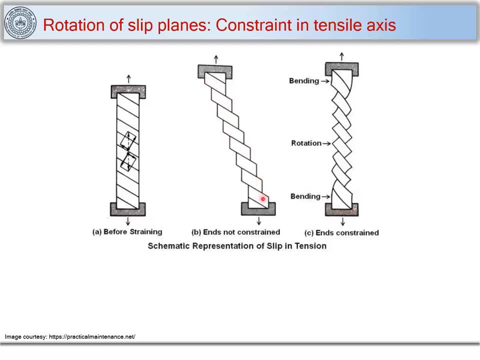 start occurring on these planes where the mid-factors are highest. So it will deform in this way. When you see a slip, A tensile test, these ends are not free to move. so here, in this case, you can see that the specimen is not or it is not allowed to deform freely, and that is what occurs in a typical tensile test. 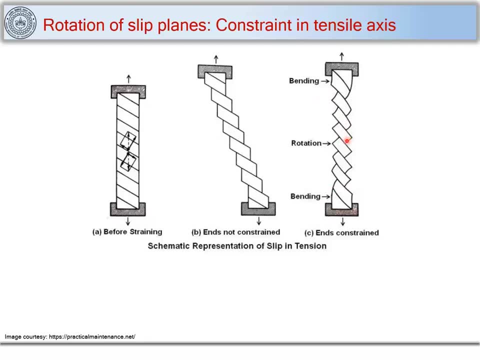 So the slip planes will try to rotate towards the tensile axis, as because the tensile axis remains fixed or constrained. So we can see that, which are the slip systems that are. So we can see that, which are the slip systems that are. 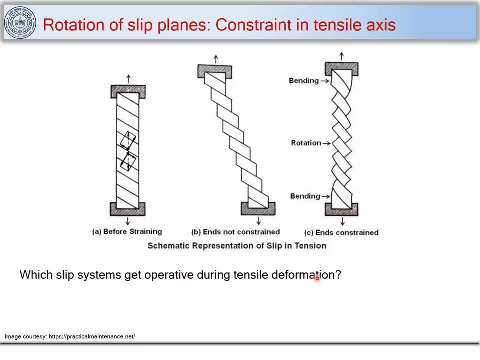 That can get operated during tensile deformation And that we can understood using a stereographic projection. So this stereographic projection is not for an exam. So, those who are interested, I would like to take an extra class to see which are the 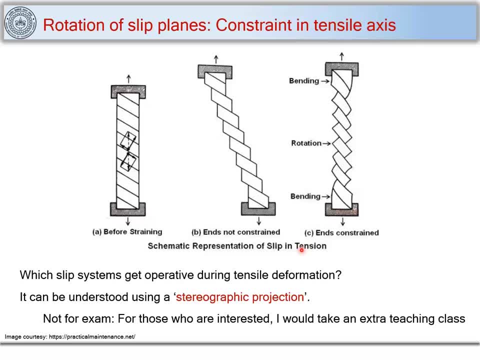 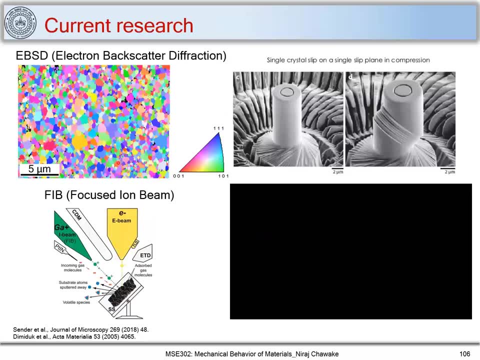 primary slip systems or secondary slip systems and how to identify slip system As we move over longer, as we Go on increasing the deformation. Now let me Tell you something about How can立ỡs� about current research in this area. So we have seen here as a single crystal So forming. 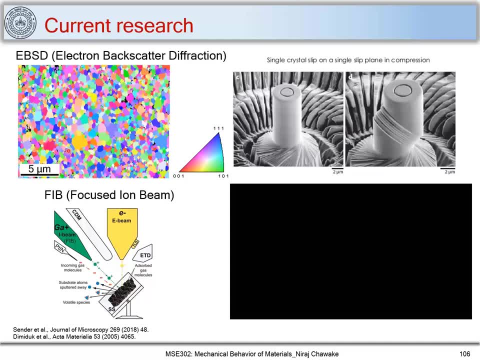 those single crystal- big single crystal- become difficult sometimes. So we can use an EBSD plot where we know the orientation of each grain and, if you have sufficiently long grains and sufficiently more area, what we can do is that each grain is representing a single 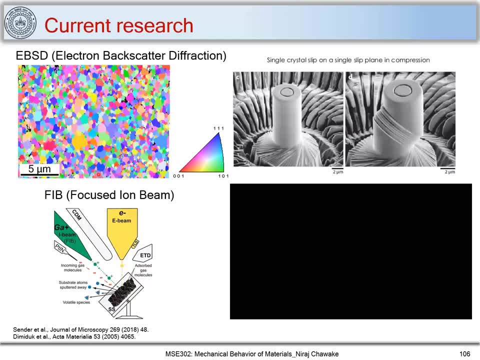 crystal. And then I can use this FIP technique and make out some pillars like this which are very small in size- You can see like these are two microns And this is a pillar before deformation and I put a small indenter on this surface and try to deform. So here you. 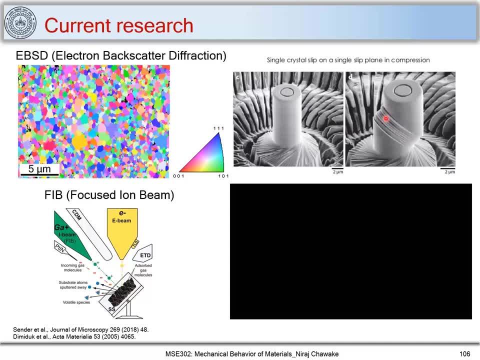 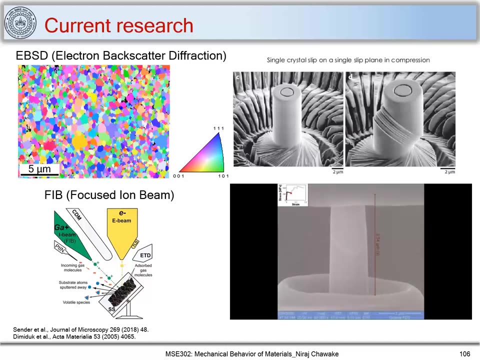 can see this single crystal is being deformed. You can see the slip is occurring on certain crystals. These are the crystallographic planes and these are the slip lines which we can see it here. Let me play a video for you. It's from Professor Greer's lab, So here you can.